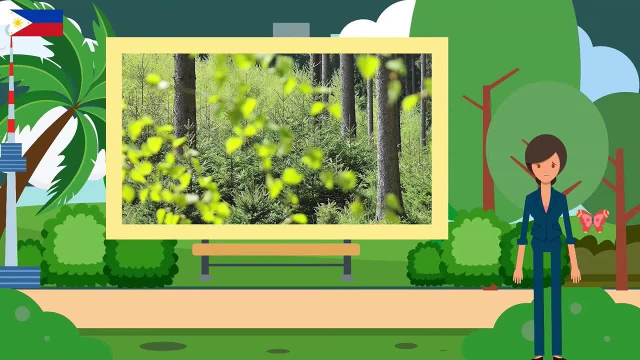 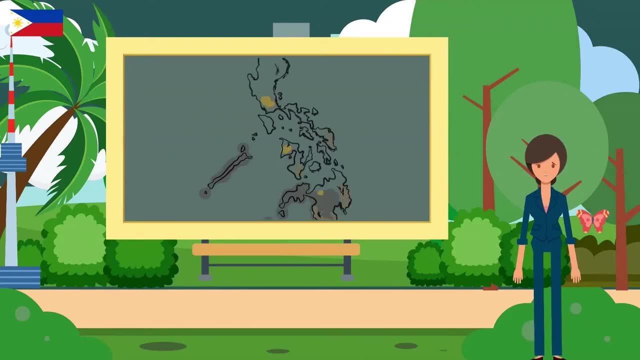 Tall grasses have replaced the forests, which have disappeared due to logging, mining and development. The Philippines are inhabited by more than 200 species of mammals, including monkeys, squirrels, lemurs, mice, pangolins, chevrotimps. 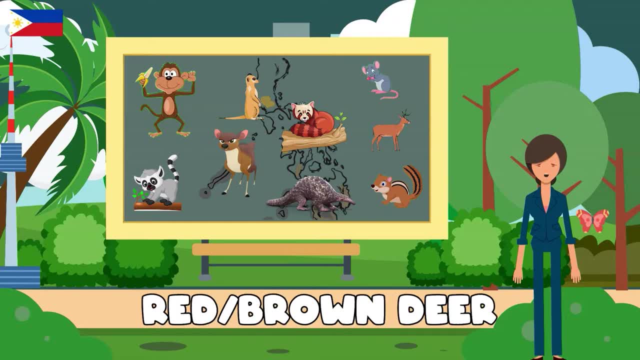 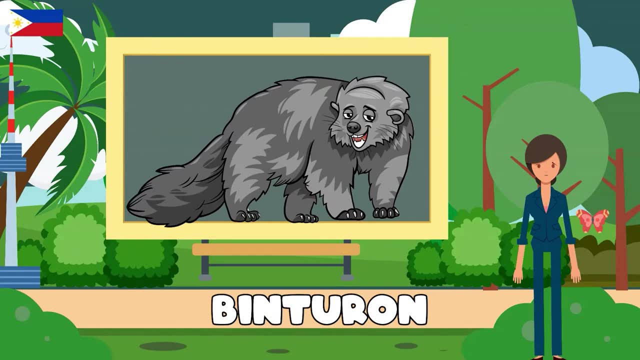 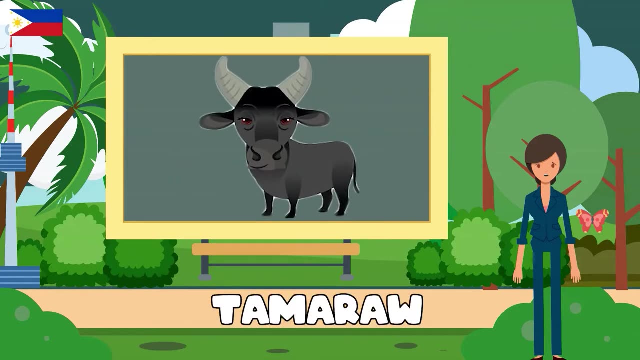 mongooses, civet cats and red and brown deer, among others. The binturon, or Asian bear cat, was once prominent, but now this furry mammal is vulnerable. The tamaraw, a species of small water buffalo found only on Mindoro, is critically endangered. 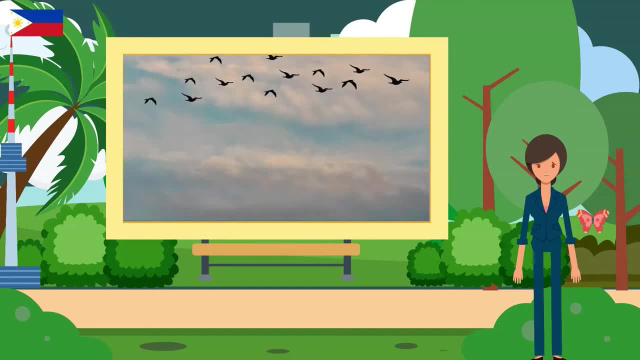 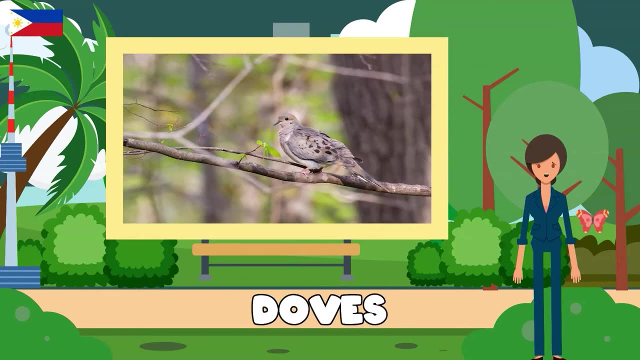 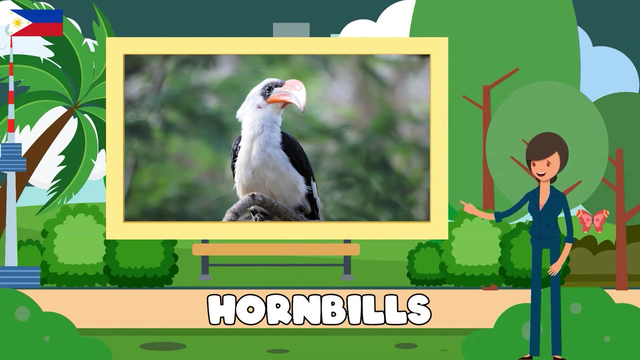 Hundreds of species of birds live in the Philippines either for all or part of the year, including peacocks, pheasants, doves, parrots, kingfishers, sunbirds, tailor birds and hornbills. The endangered Philippine eagle, which eats monkeys, is barely surviving deforestation. 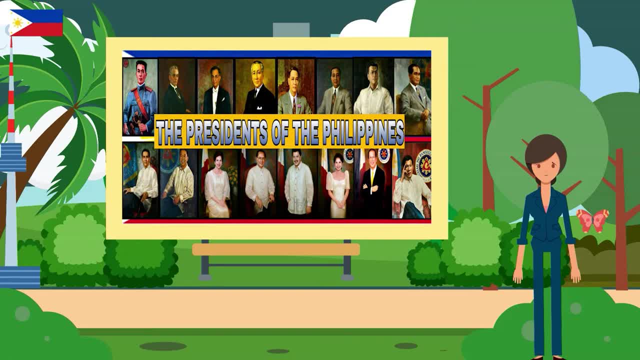 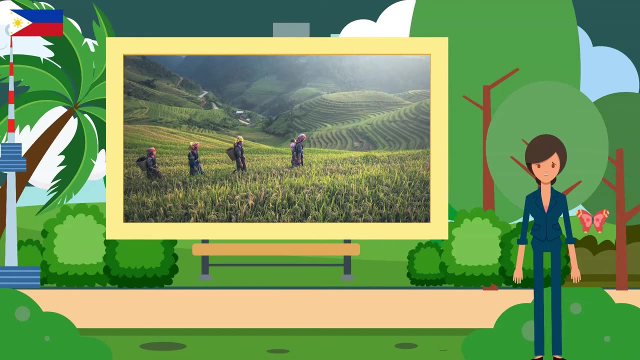 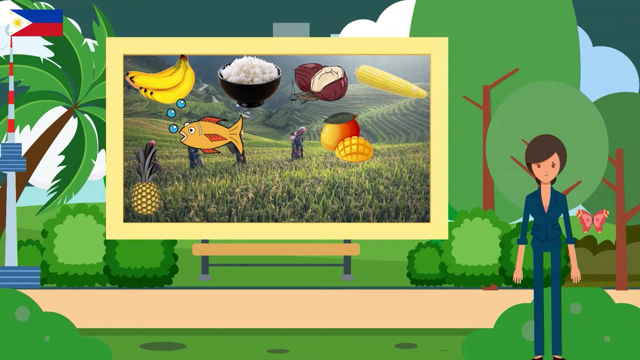 Filipinos elect their president. The president is the head of state. The president is the commander-in-chief of the armed forces and serves a six-year term. The economy is based on agriculture, light industry and services. The country produces bananas, rice, coconuts, corn, fish, mangoes, pineapples, sugarcane, pork and beef. 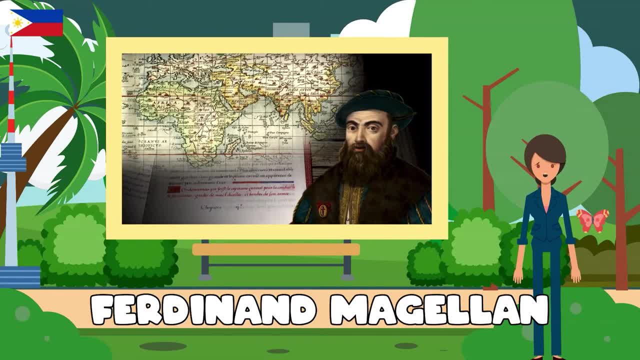 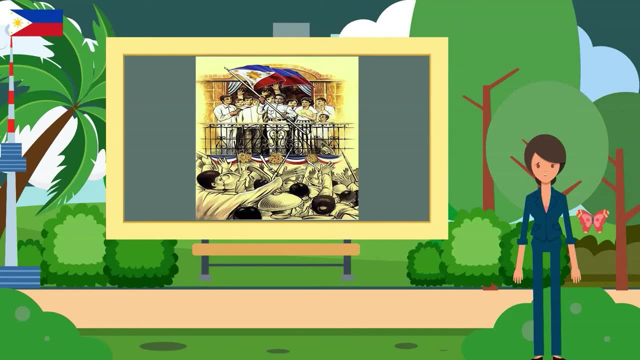 Ferdinand Magellan first landed in the Philippines in 1521.. The name Philippines comes from the name of the Philippines. The name Philippines comes from the name of the Philippines. Its name indicates the sportive and active behavior ofDIES inaga. The name Philippines comes from Philip II, who was the King of Spain during the 16th century, when the country became a Spanish colony. 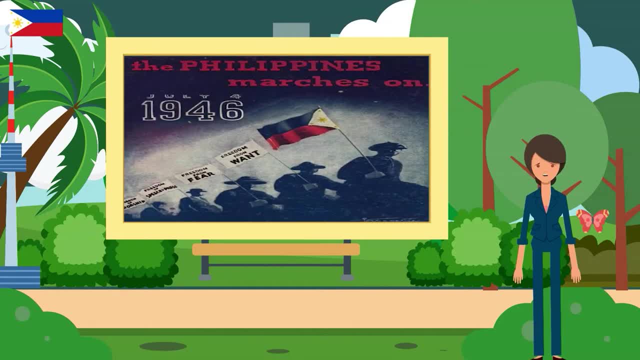 The Philippines was granted the United States in 1898, following the Spanish–American War In 1935, the Philippines became self-governing, but their independence was delayed by World War II and the invasion of Japanese troops. The Philippines's independence was delayed by World War I and the invasion of Japanese troops.